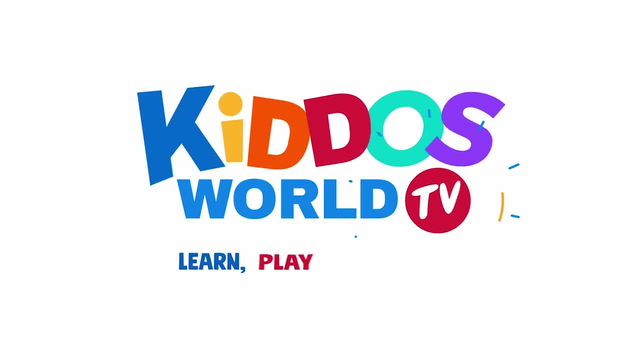 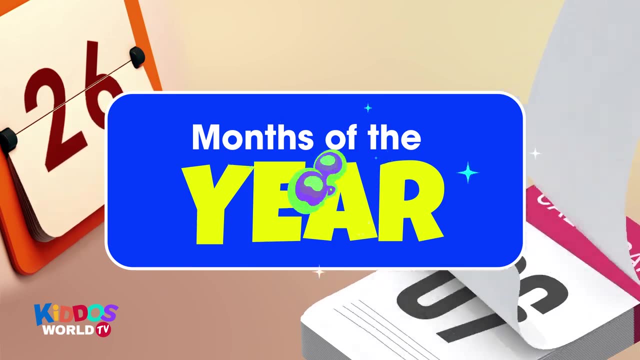 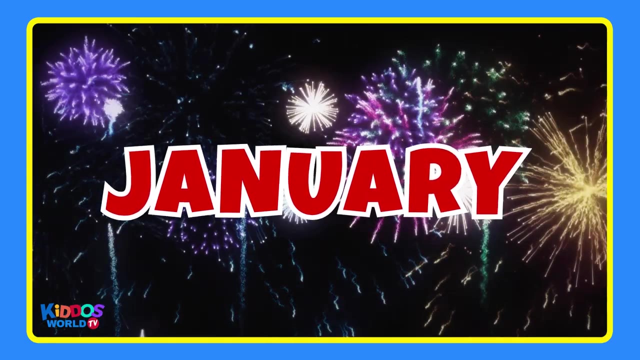 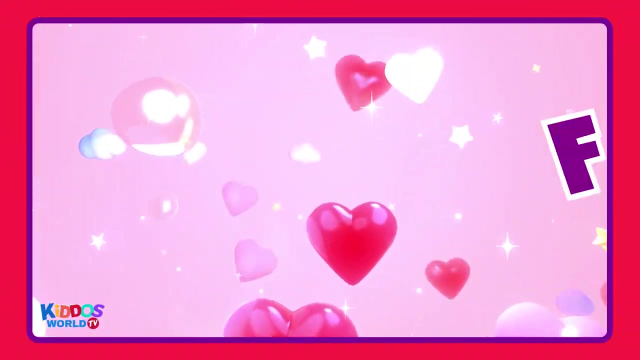 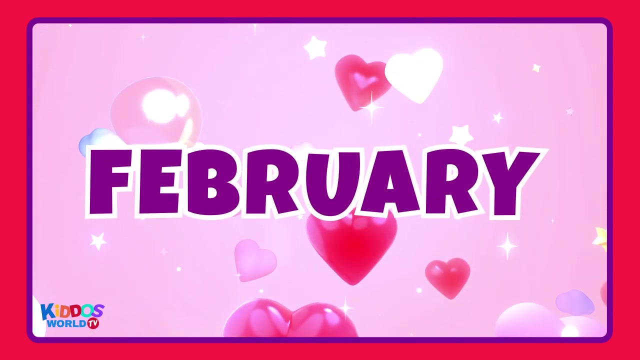 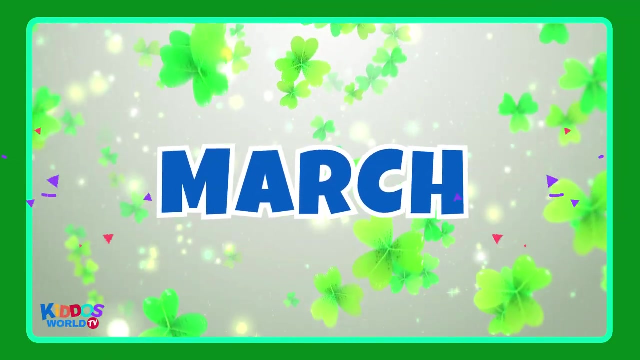 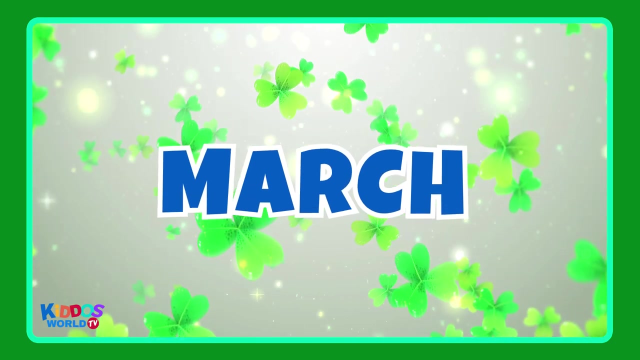 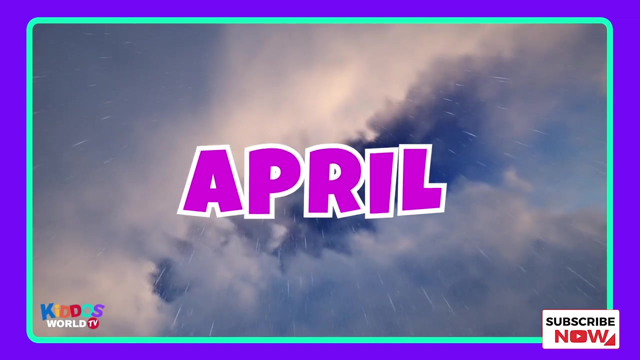 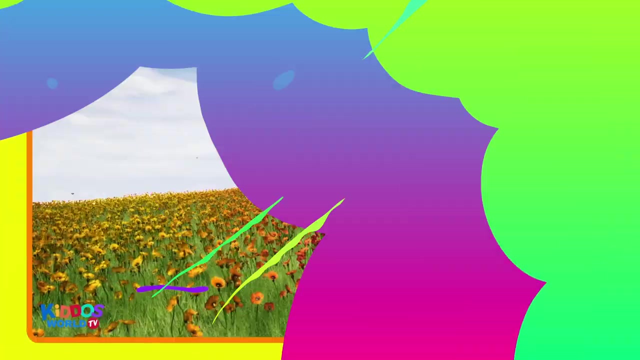 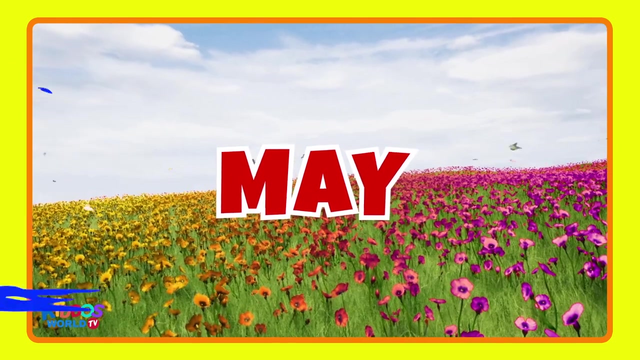 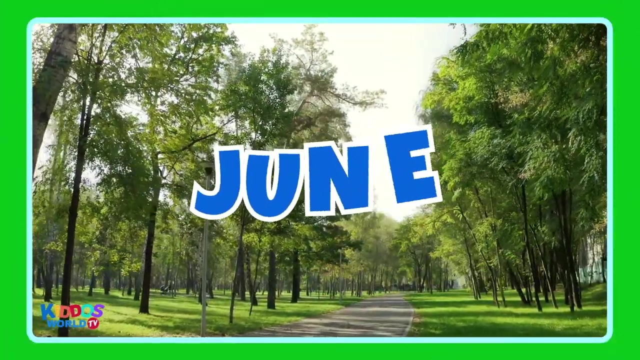 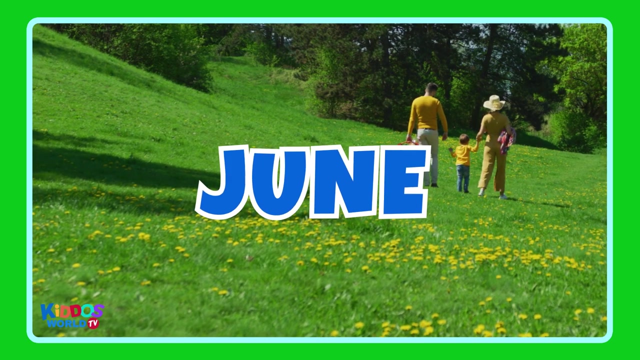 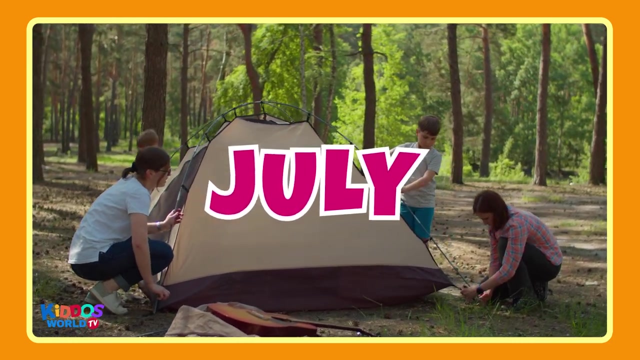 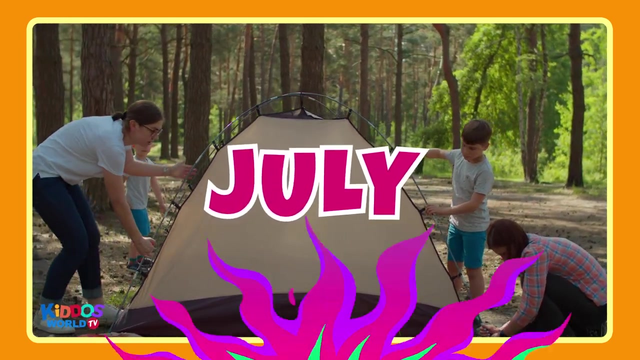 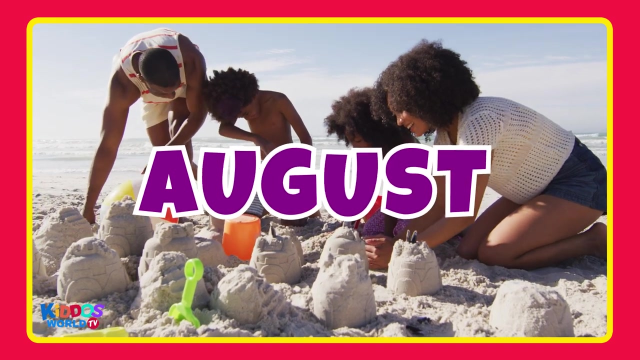 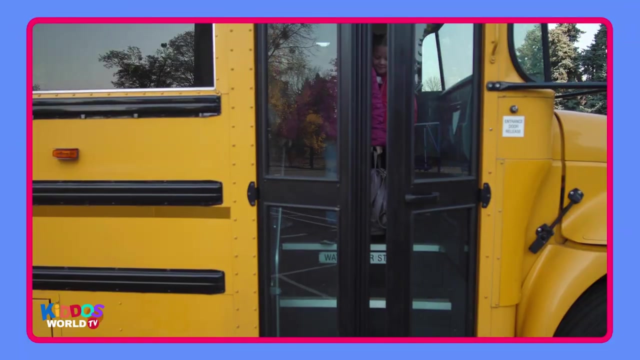 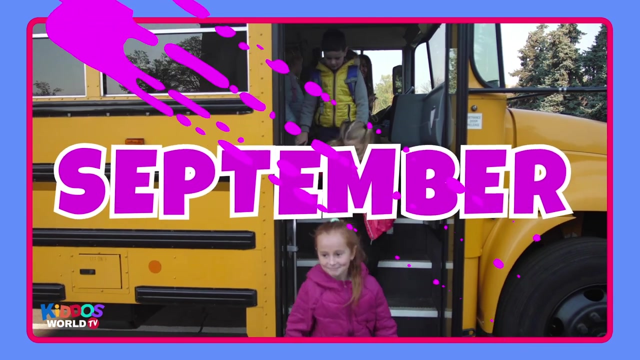 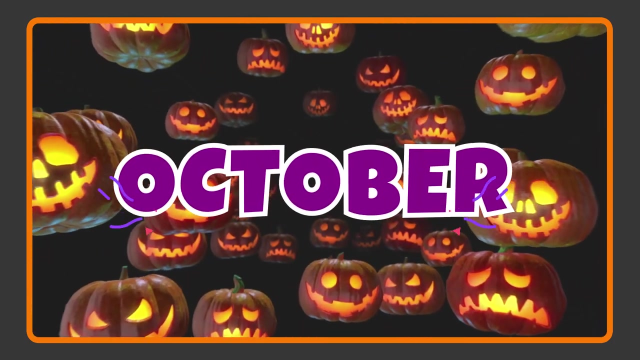 You're watching Kiddos World TV. Hi, kiddos, Let's learn the months of the year. Here we go: January, January, February, February, March, March, April, April, May, May, May, June, June, July, July, July, August, August, September, September, July, October, October, October, October. 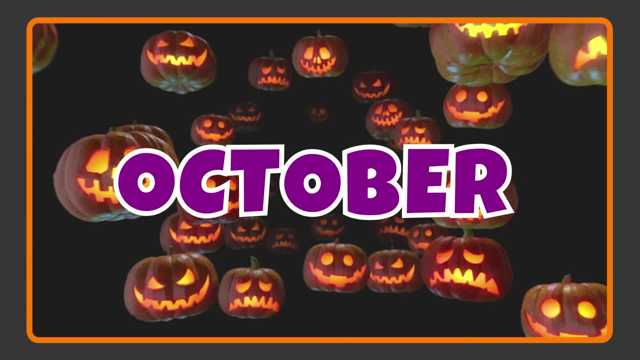 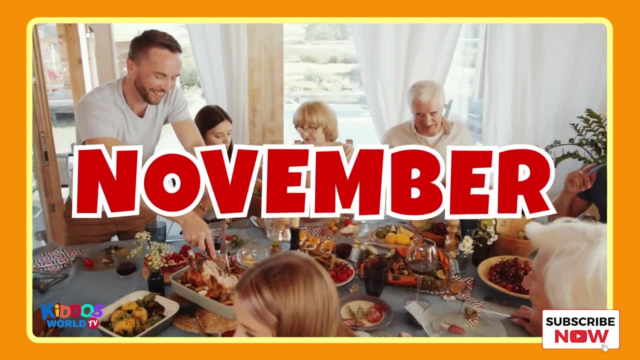 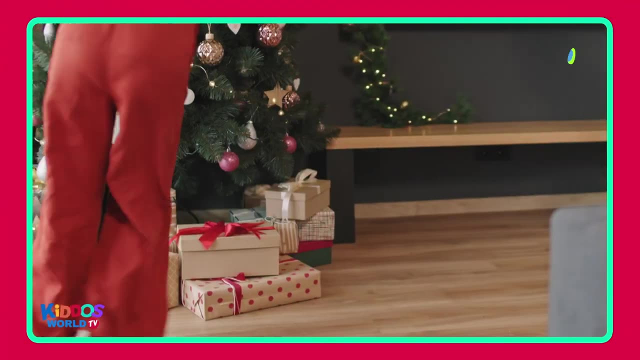 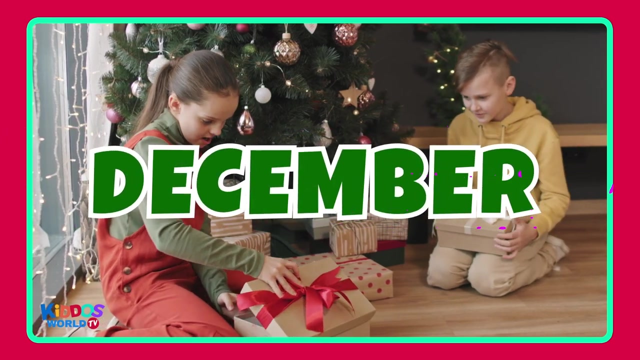 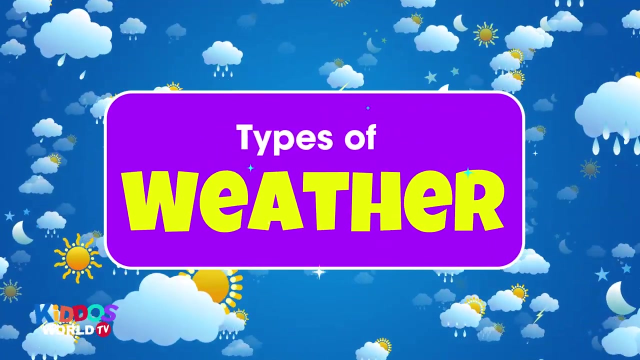 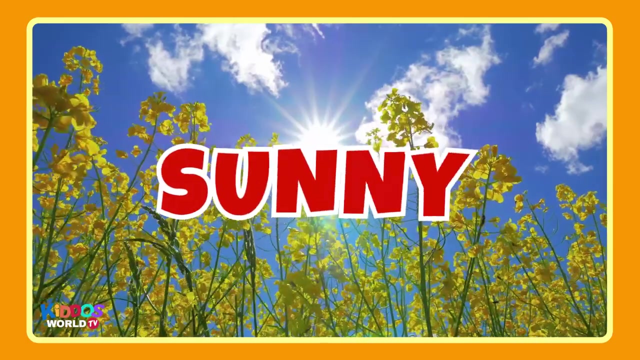 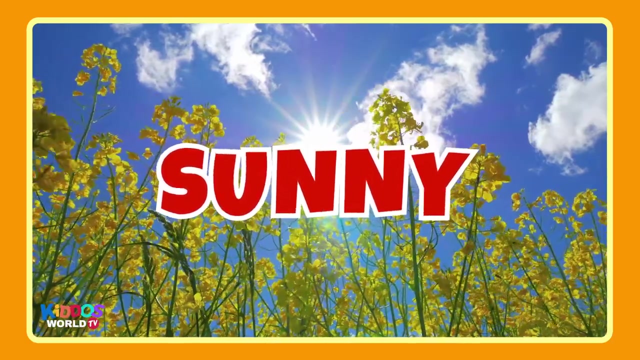 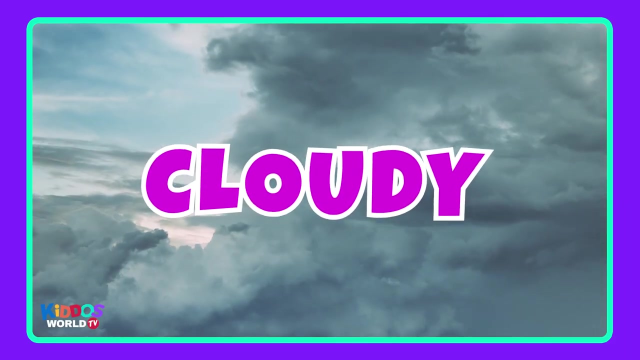 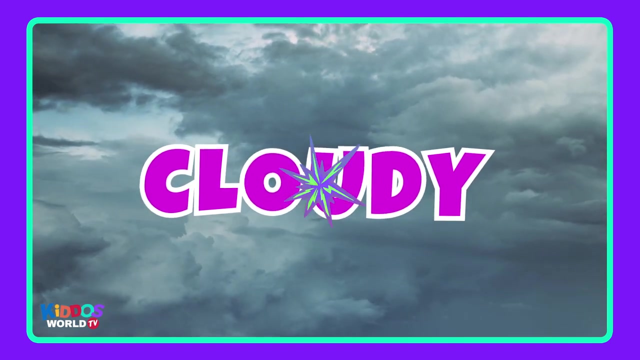 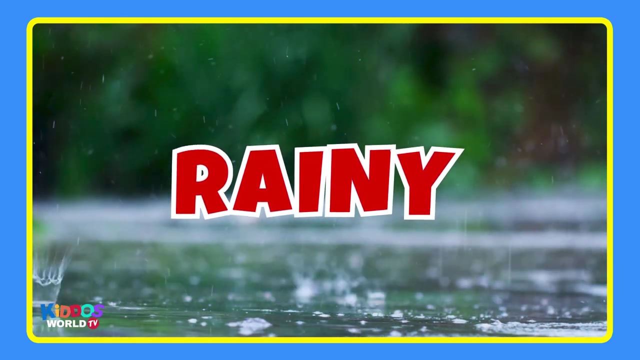 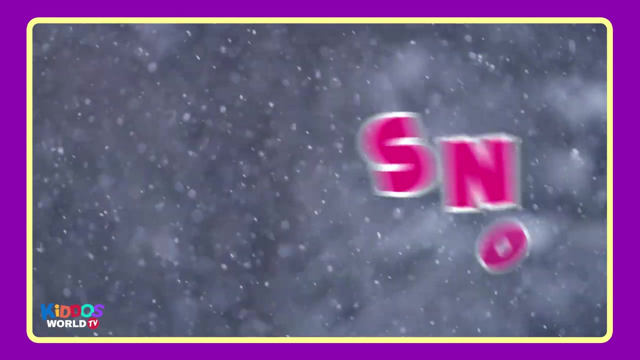 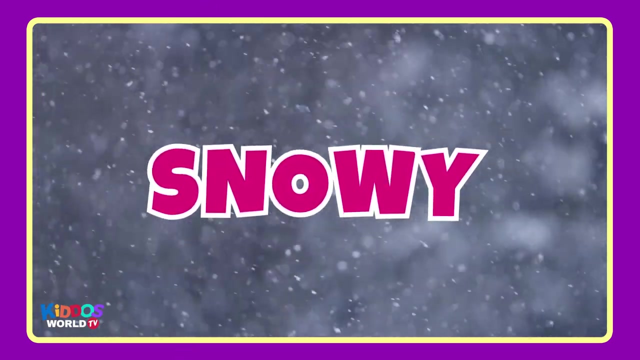 October, November, November, December. Let's go to the next one. Hi, kiddos, Let's identify the different kinds of weather. Here we go: Sunny, Sunny, Cloudy, Cloudy, Rainy, Rainy, Snowy, Snowy. 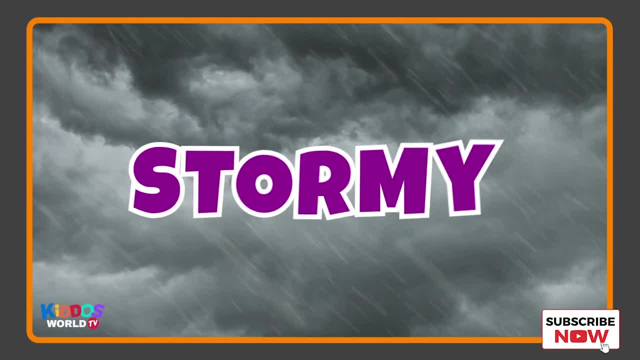 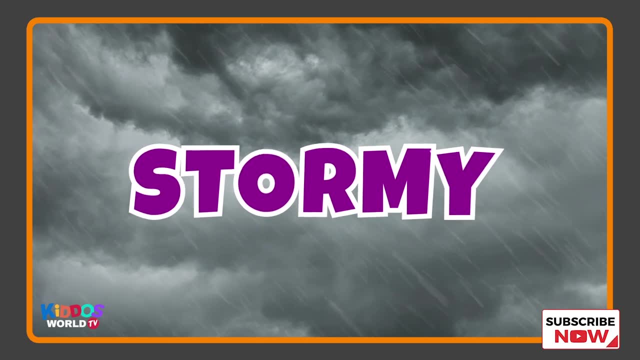 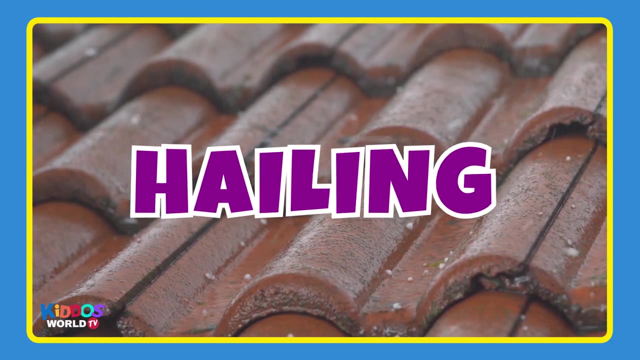 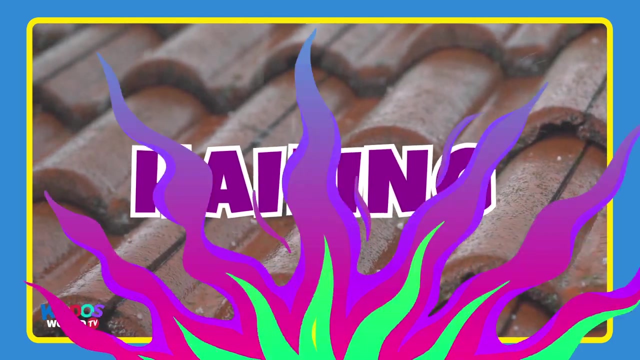 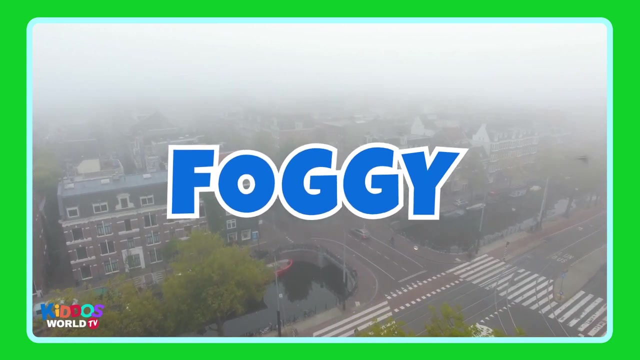 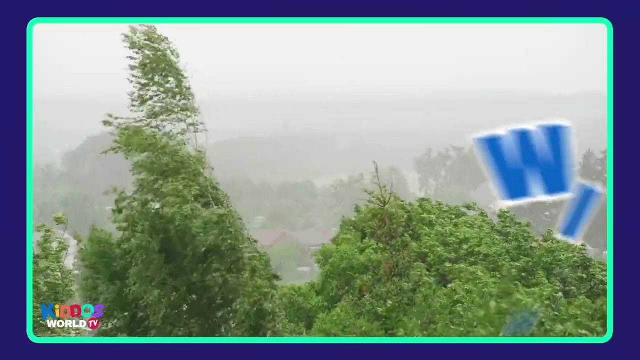 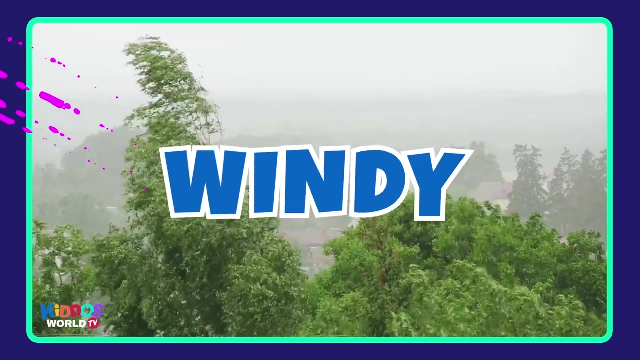 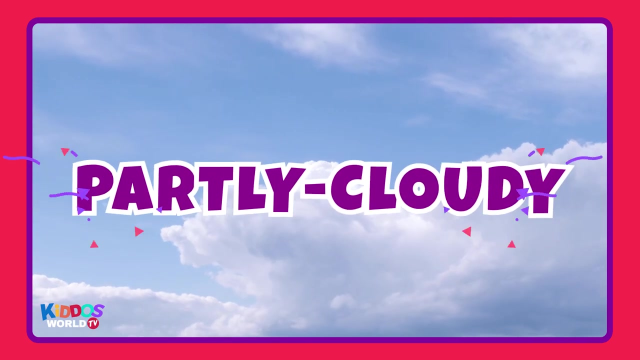 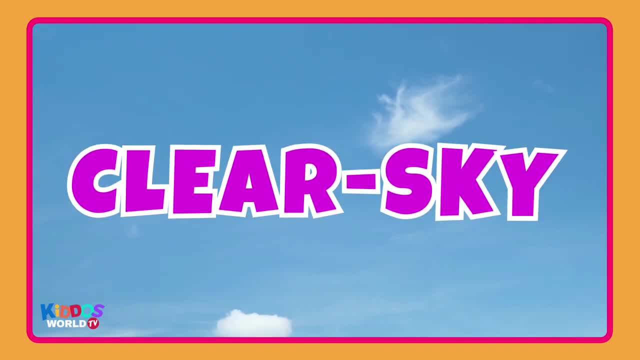 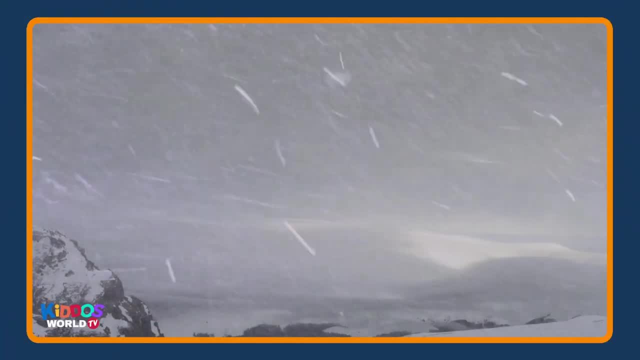 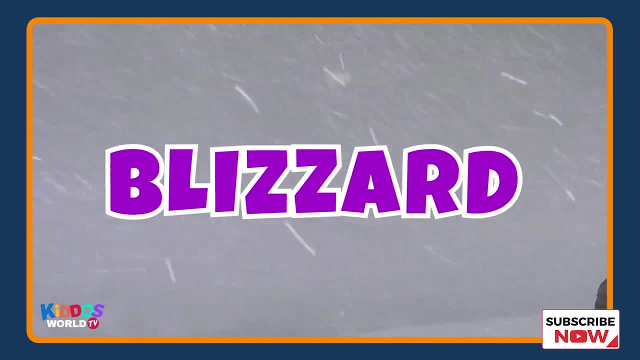 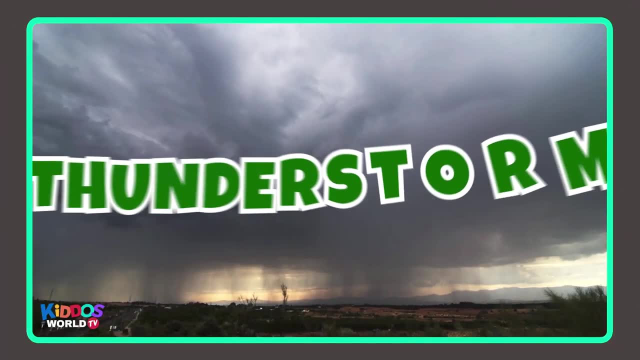 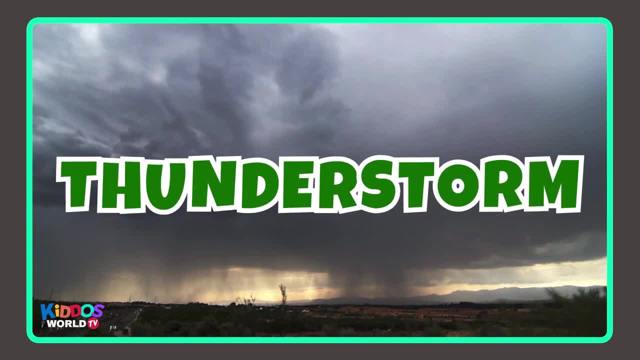 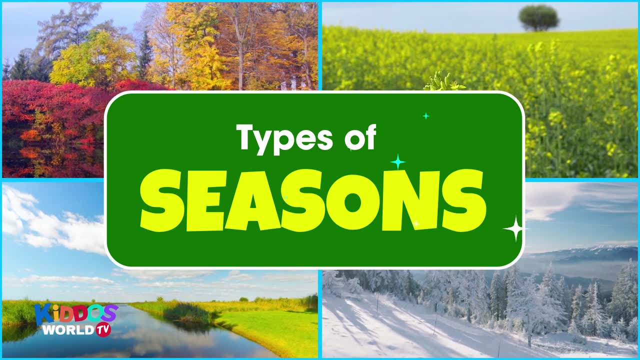 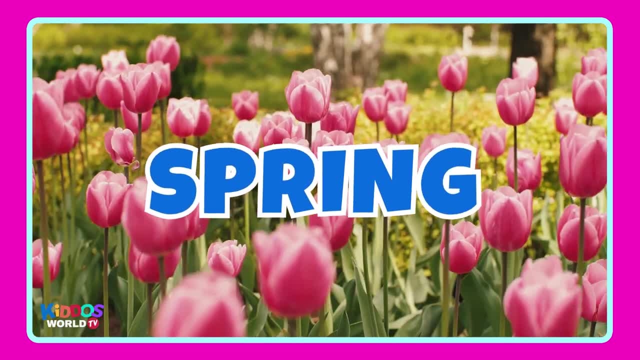 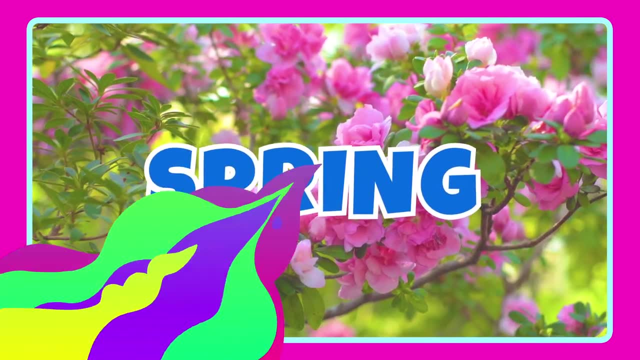 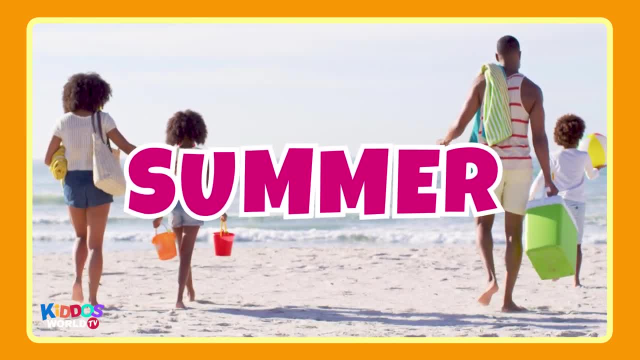 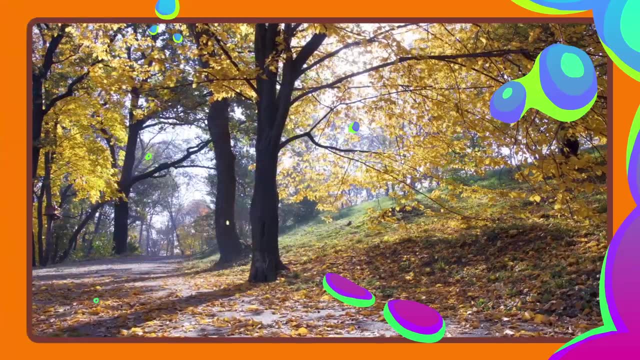 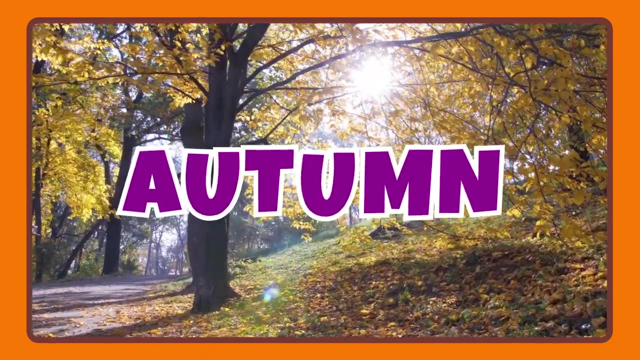 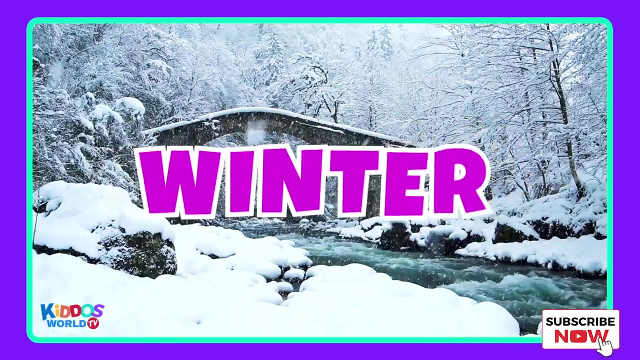 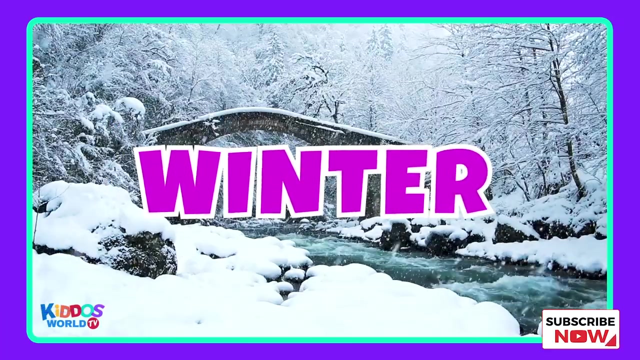 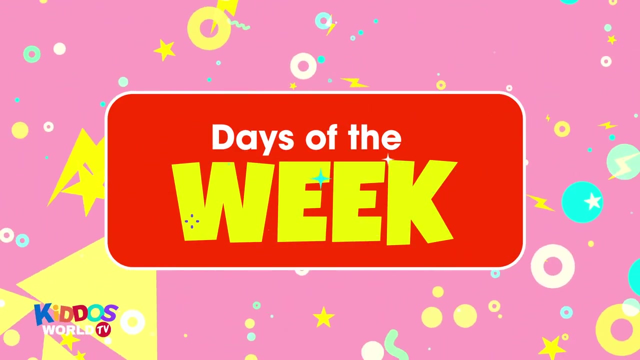 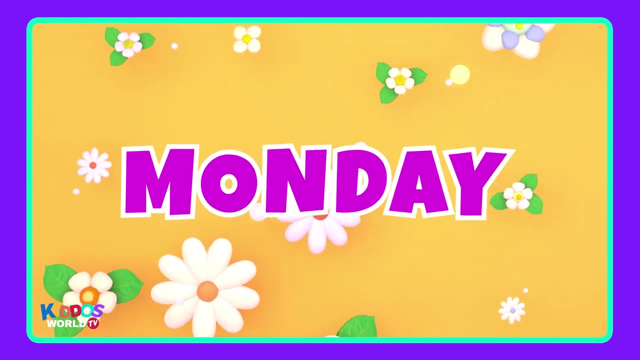 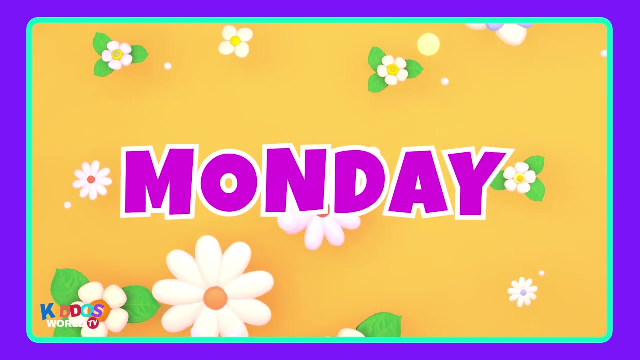 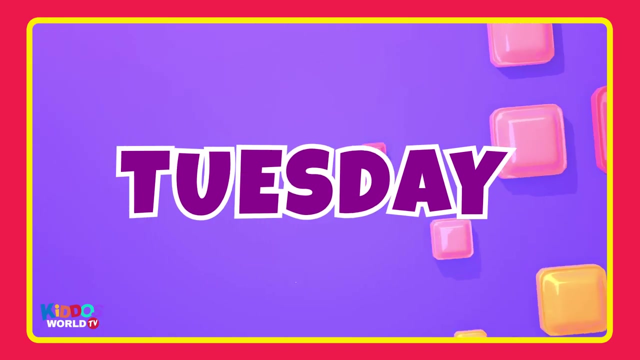 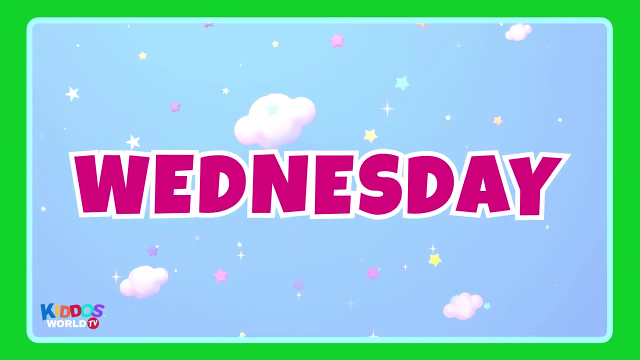 Partly cloudy, Partly cloudy, Partly cloudy. Surprise, Summer, Autumn, Autumn, Winter, Winter. Let's go to the next one. We're going to learn about the days of the week. Say it with me: Monday, Monday, Tuesday, Tuesday, Tuesday, Wednesday, Wednesday. 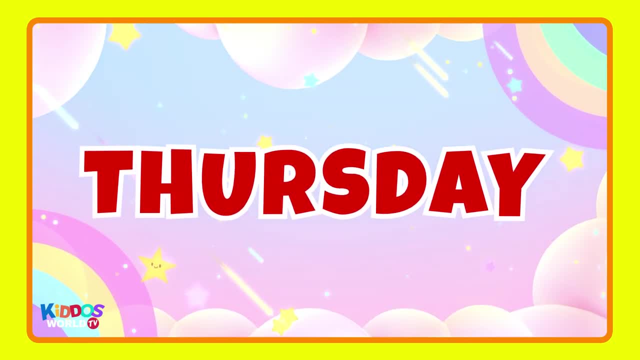 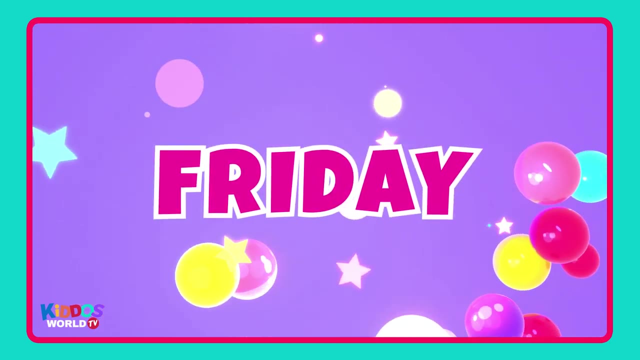 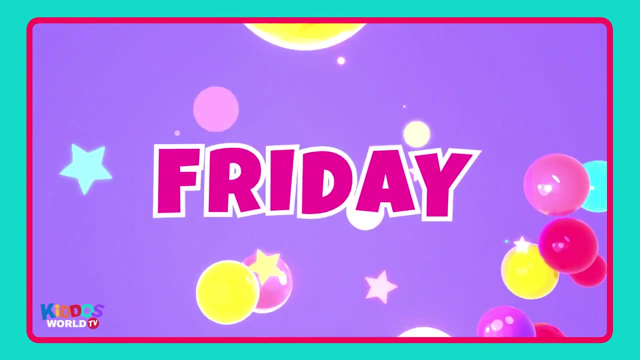 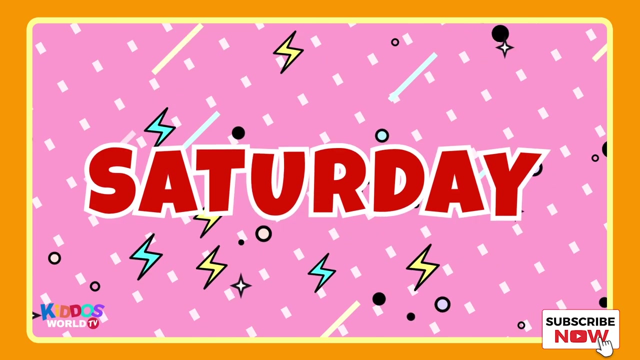 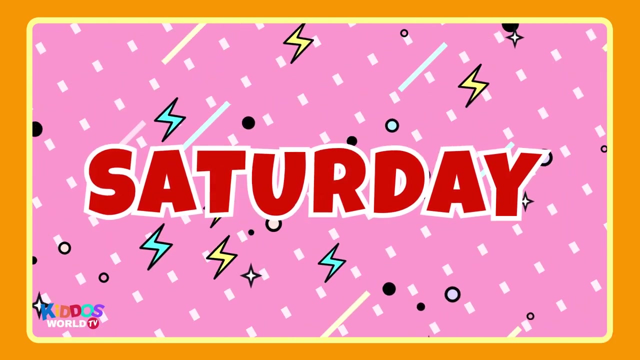 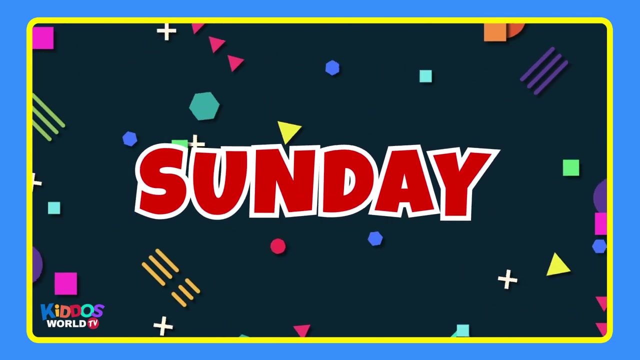 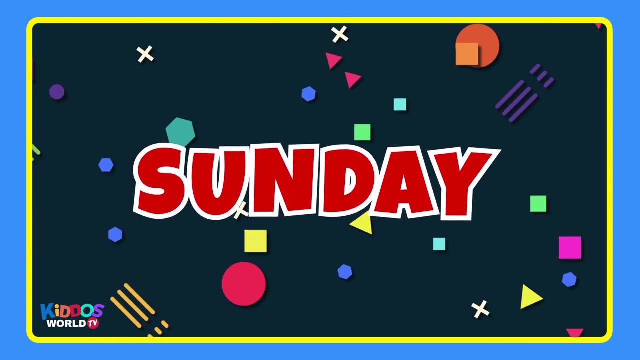 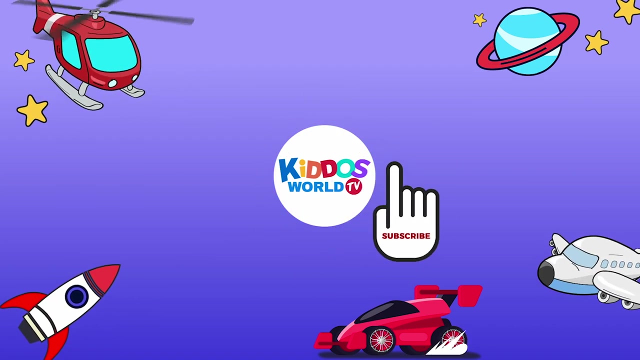 Thursday, Thursday, Thursday, Friday, Friday, Saturday, Saturday, Saturday, Sunday, Sunday, Bravo, Great work. kiddos Having fun. kiddos, Please click subscribe for more learning and fun. See you in the next videos. Thank you.